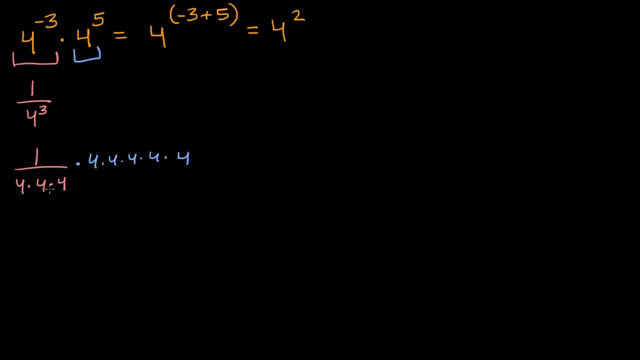 and three fours in the denominator, And so three of these in the denominator are going to cancel out with three of these in the numerator, And so you're going to be left with five minus three or negative three plus five fours. So this four times four is the same thing as four squared. 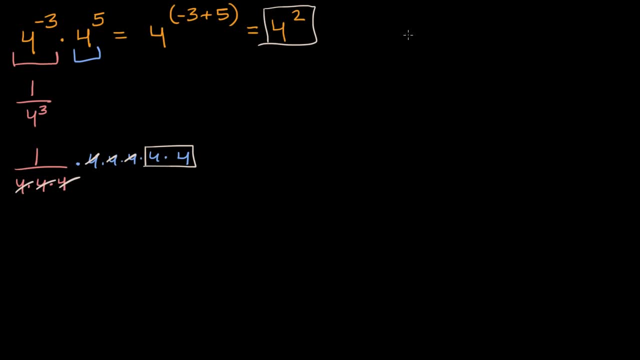 Now let's do one with variables. So let's say that you have a a to the negative, four power times a to the, let's say a squared. What is that going to be? Well, once again, you have the same base. in this case it's a and so, since I'm multiplying them, 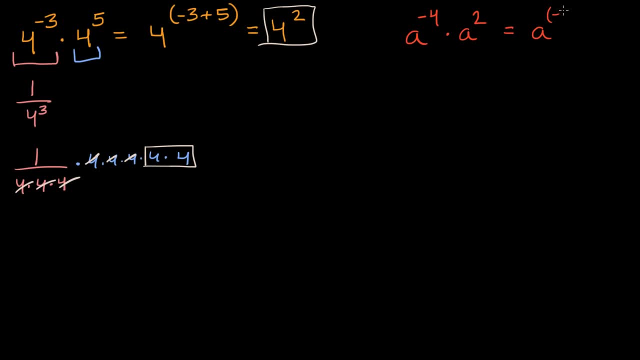 you can just add the exponents, So it's going to be a to the negative four plus two power, which is equal to a to the negative two power, And once again it should make sense This right over here, that is one over a times a. 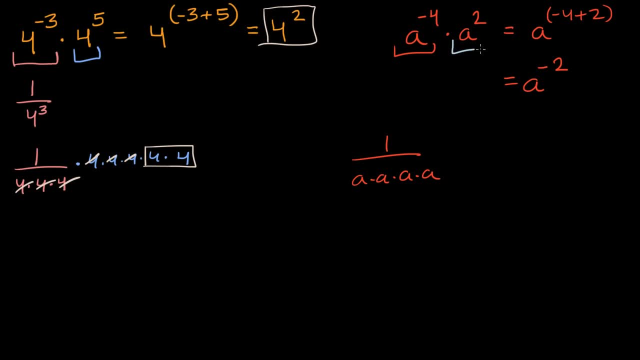 times a times a, and then this is times a times a. So that cancels with that, that cancels with that, and you're still left with one over a times a, which is the same thing as a, to the negative two power. 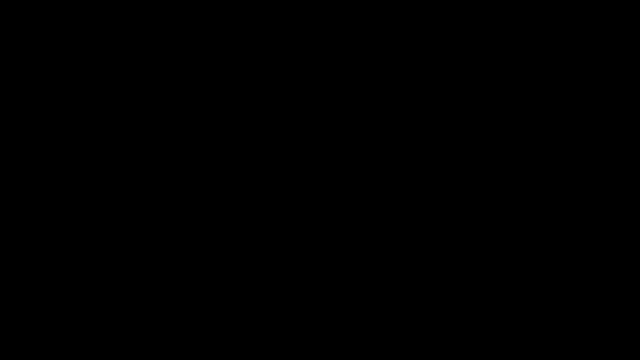 Now let's do it with some quotients. So what if I were to ask you: what is, what is? what is 12 to the negative seven divided by 12 to the negative five power? Well, when you're dividing, you subtract exponents. 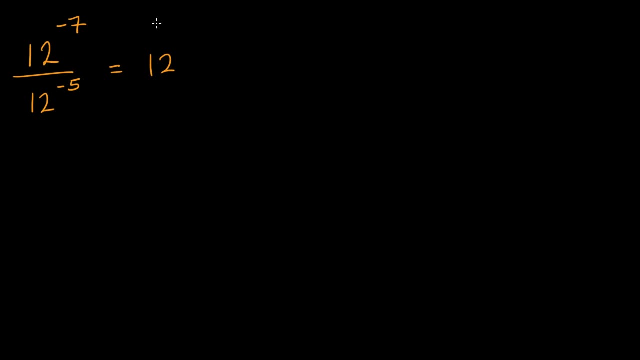 If you have the same base. So this is going to be equal to 12 to the negative seven minus negative five power. You're subtracting the bottom exponent And so this is going to be equal to 12 to the well that. 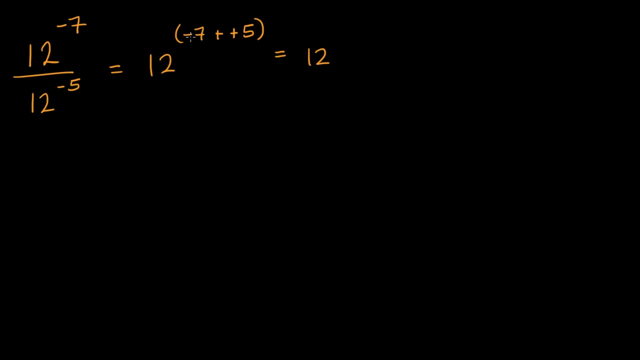 Subtracting a negative is the same thing as adding the positive A 12 to the negative two power. And once again we just have to think about why does this actually make sense? Well, you can actually rewrite this: 12 to the negative seven divided by 12 to the negative five.